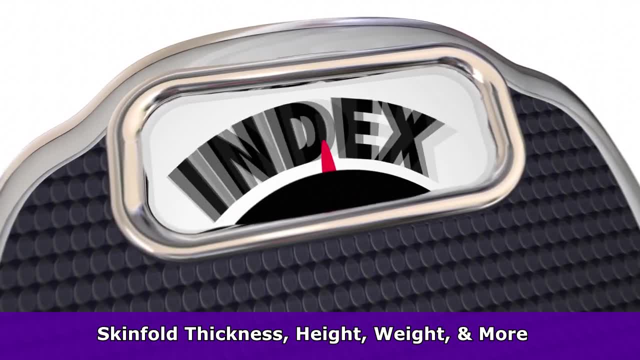 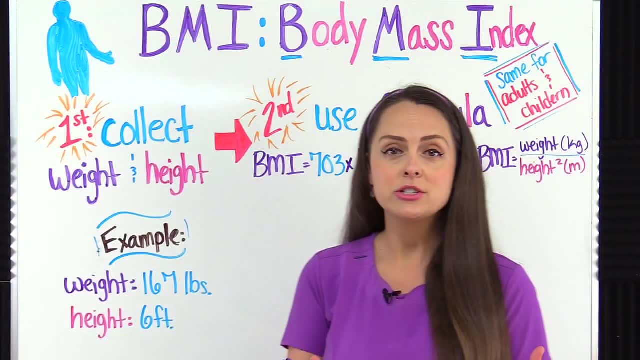 such as skinfold thickness, height, weight and so on. Now, BMI scores are really helpful because they allow us to screen patients for potential health problems. So in this video, I'm going to show you how to calculate this number manually. So first, what you want to do is you want to. 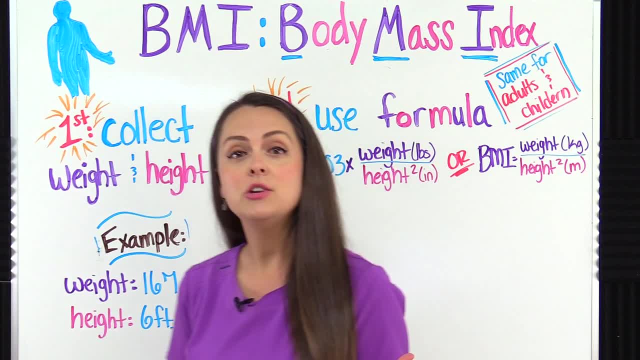 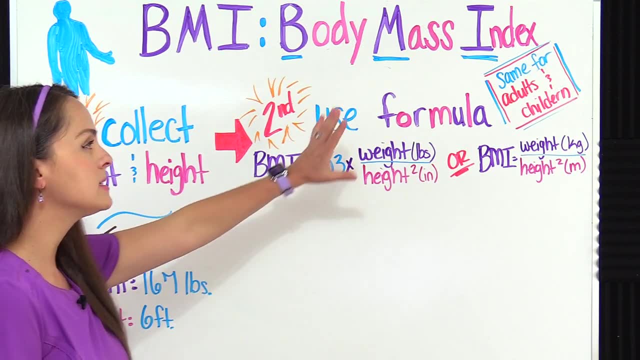 collect the patient's weight and height. Then, once you have that, you want to use a formula and plug in the information you have into whatever formula you want to use. Now, the formula that you use is the same for adults and children, male or female, but it depends on which measurement. 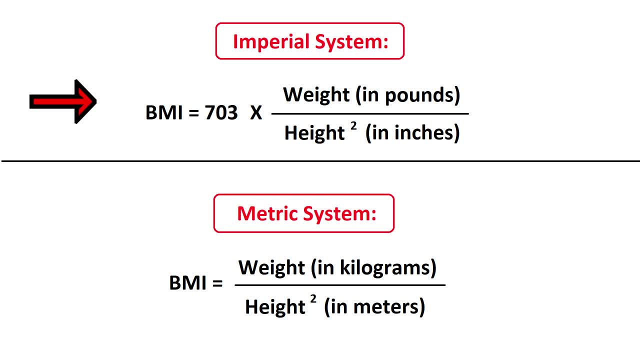 system you're using. For example, if you're using the imperial system, such as pounds and inches, you're going to use this formula, But if you're using the metric units, like kilograms of meat, you would use this formula. So, first, what we're going to do is we're going to use this formula. 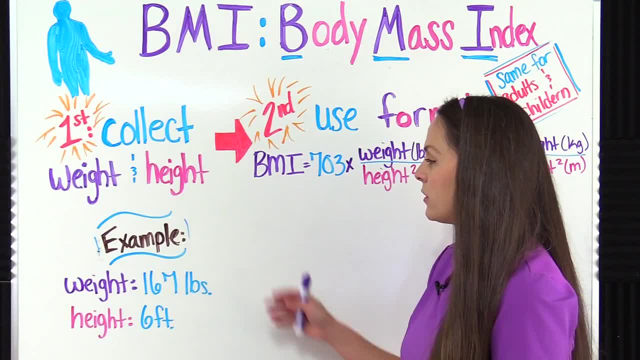 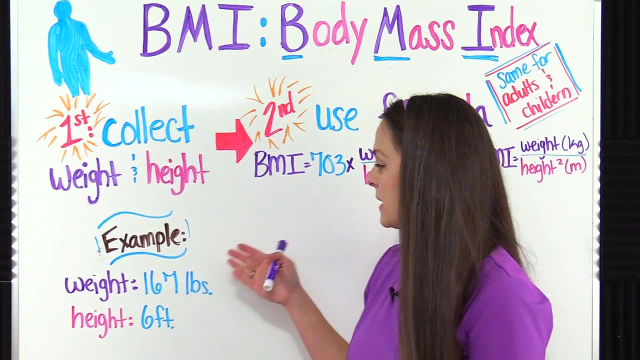 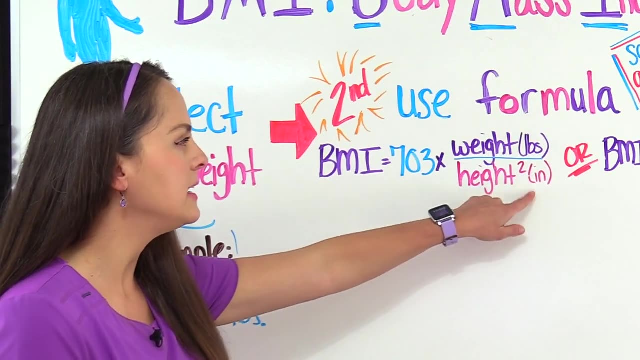 because our example over here is in imperial units, So here our patient weighs 167 pounds and they have a height of 6 feet. And because we're dealing with pounds and feet, we can use this formula right here. But notice, in this height part it needs to be an inches. So quickly what we 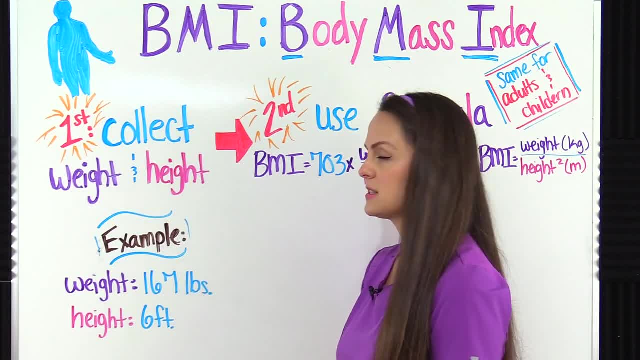 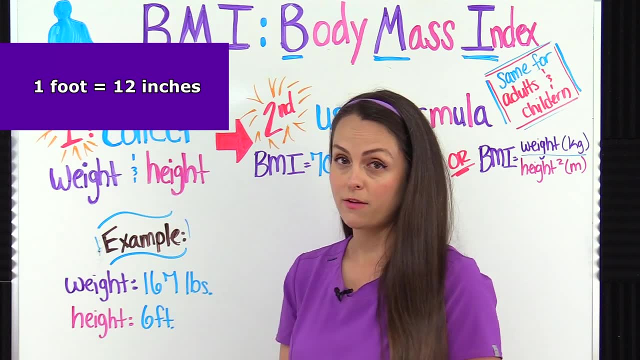 need to do is we need to convert 6 feet into inches, And to do that, you want to ask yourself how many inches are we going to be using? are in one foot? well, we know that there are 12 inches in one foot, so what we're? 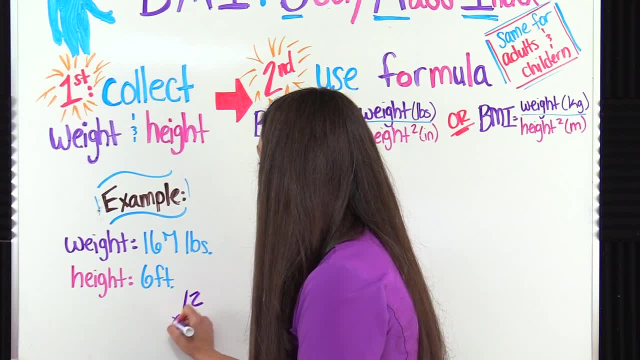 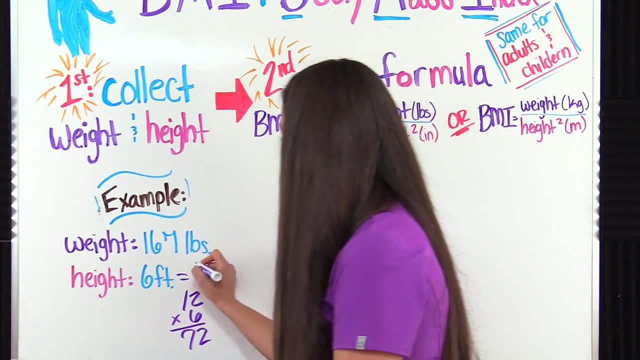 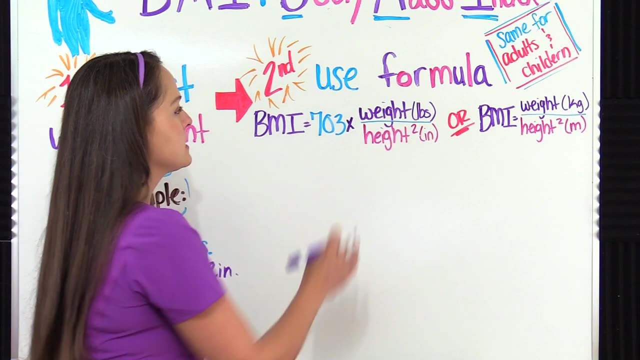 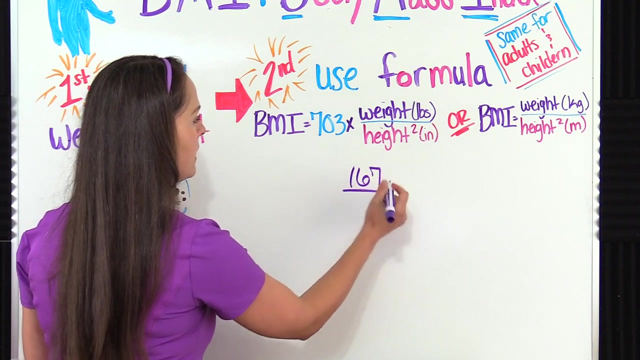 going to do is we're going to multiply 12 by 6 and that gives us 72. so 6 feet is equivalent to 72 inches. now we are ready to use our formula. so first let's plug in our weight, which was 167 pounds, so 167, and we are going to divide that. 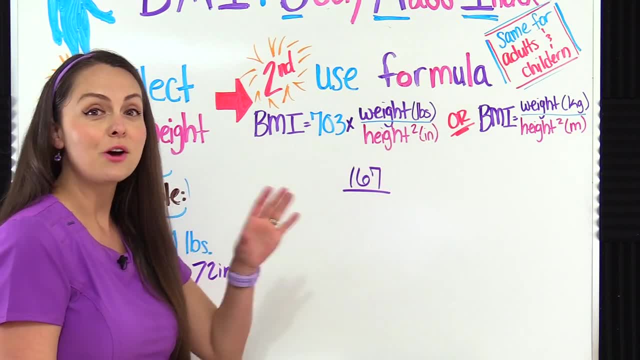 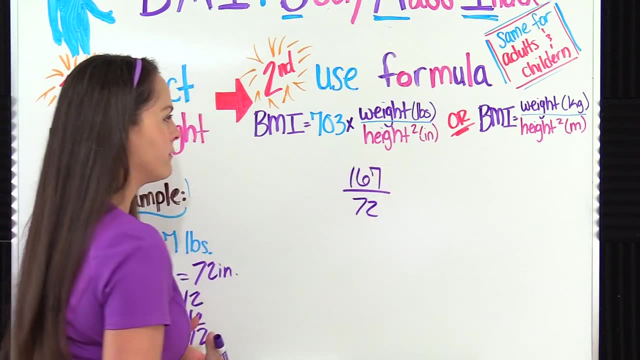 into the height in inches, but it's going to be squared, so don't forget to bring down your square part, because that's the part you could easily forget. so we're going to put in 72 inches. that's what we just figured out with our conversion and 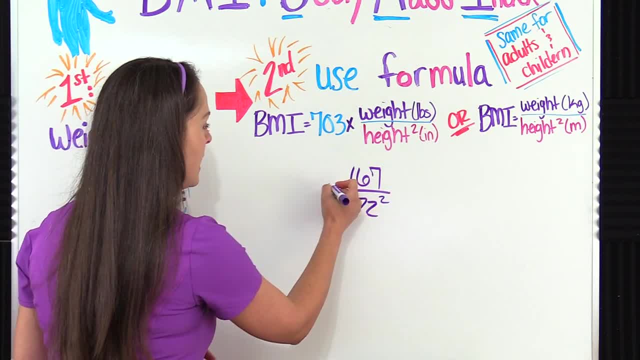 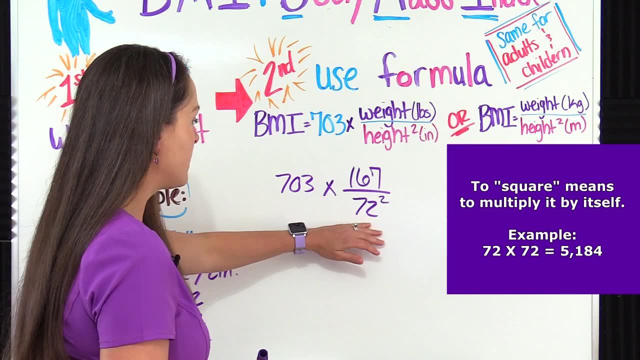 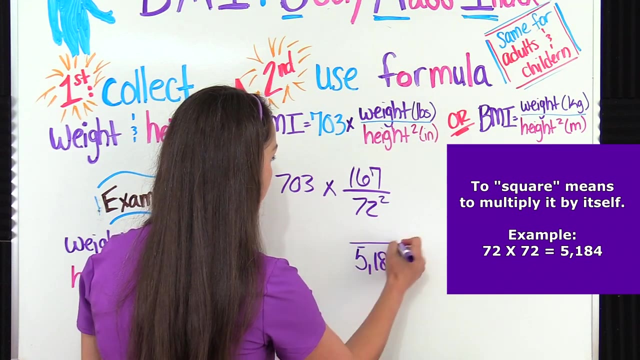 we're going to square that, so we're gonna put a little two there to remind us. we're going to multiply that by 703, so let's go ahead and square this out. when we say 72 squared, that gives us 5184. I'm going to put 167 up there, bring. 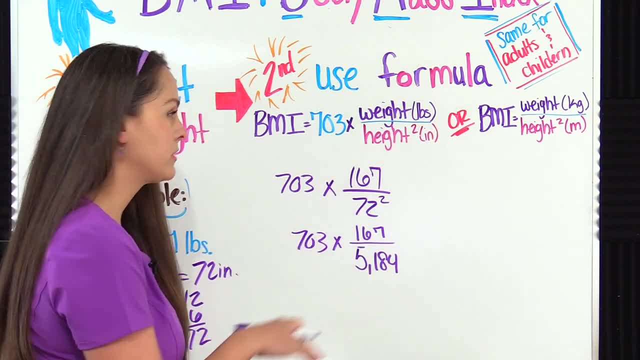 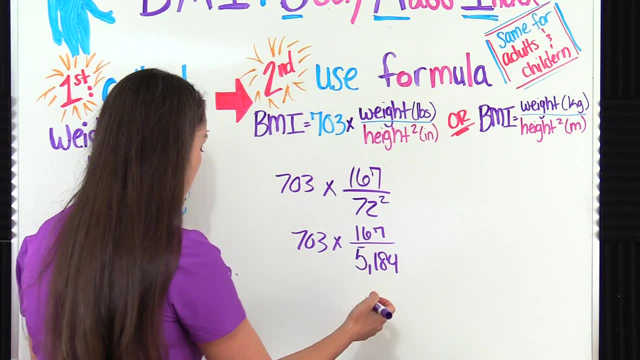 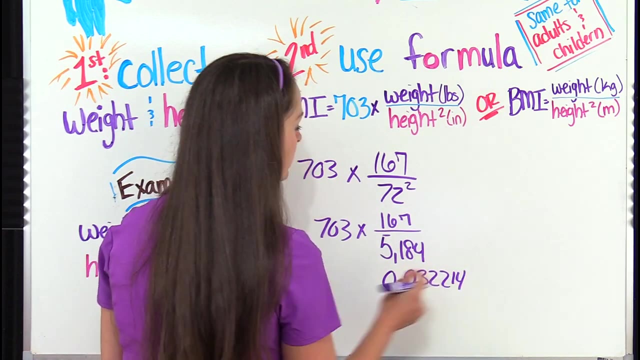 that down. so we don't forget our little 703, because I would really throw off our equation. so 167 divided by 5184, that gives us 0.032214, and it literally keeps going on. so we're going to round to the fourth decimal point, which is the ten. 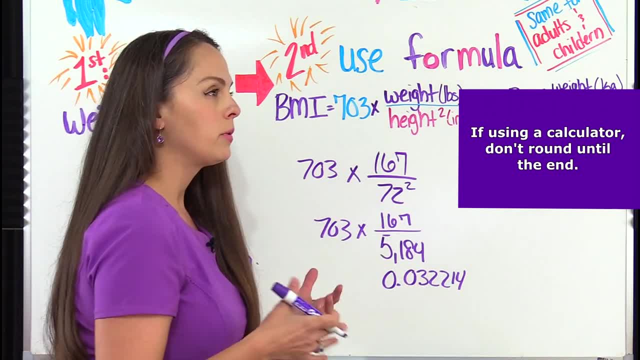 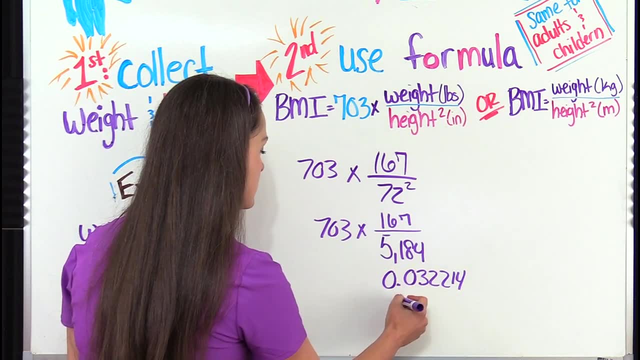 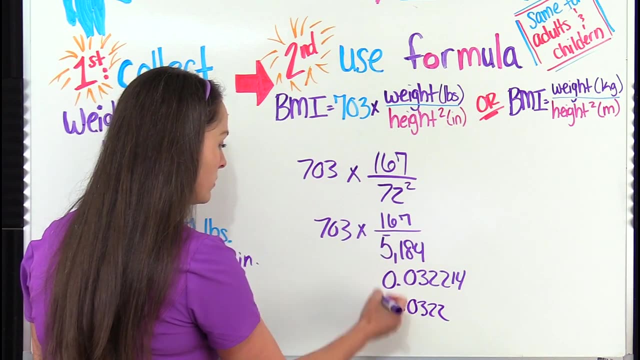 thousandths place. now round how your professor wants you to round. so follow their rounding rules. but we're going to round to the fourth decimal place, which will give us 0.0322. makes things a little bit simpler. and then we're going to multiply that by 703. so when we multiply all that out, we get 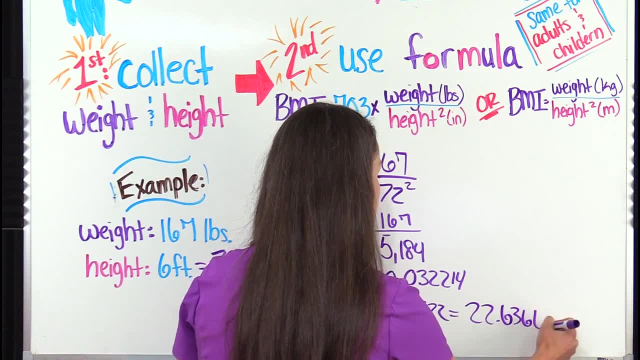 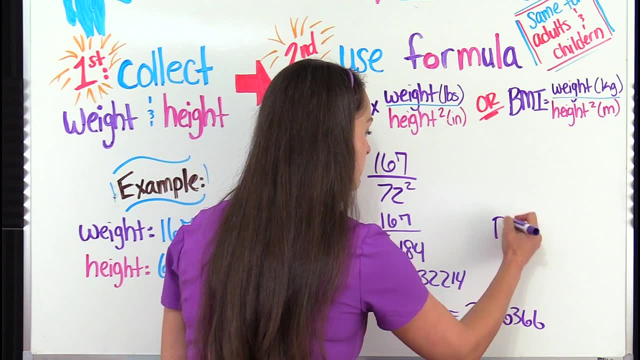 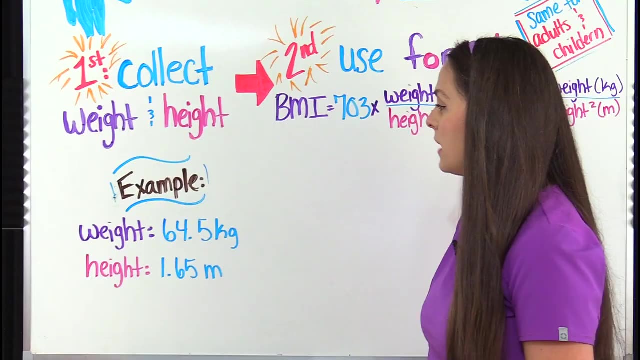 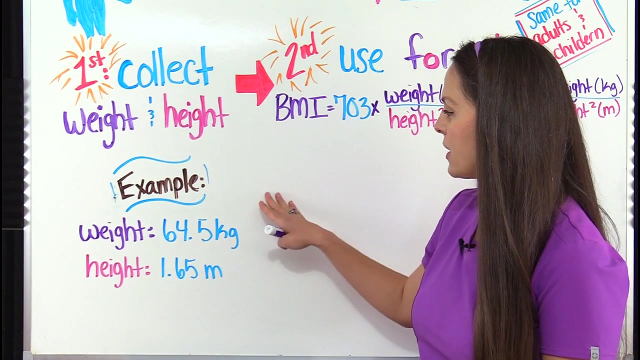 2.6366, and we're going to round our BMI to that first decimal place, which is the tenths place, and whenever we do that we get a BMI of 22.6 and that is our answer. our next patient weighs 64.5 kilograms and they have a height of 1.65 meters, so 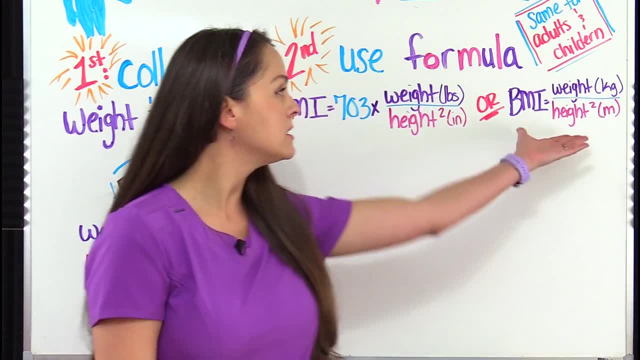 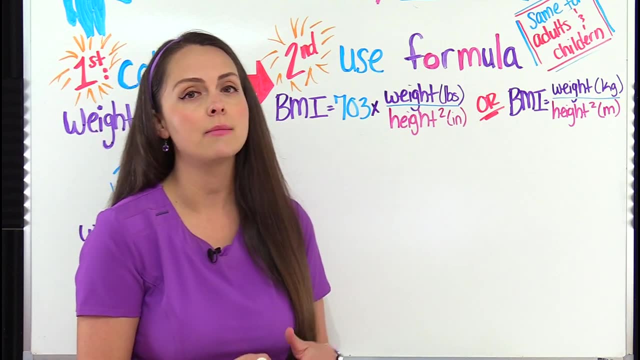 we're dealing with kilograms and meters. therefore, we can use this formula right here, which is in the metric units, and notice this formula is a little bit different than this one because we don't have to multiply by 703, so that's one less step that we have to take, so it's a little bit more simpler. 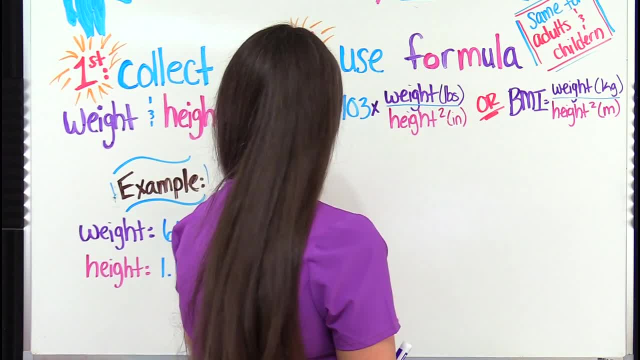 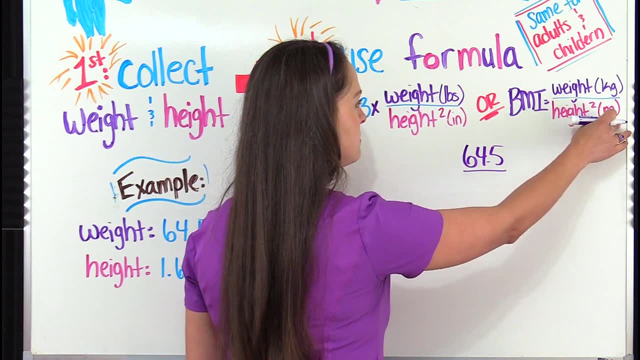 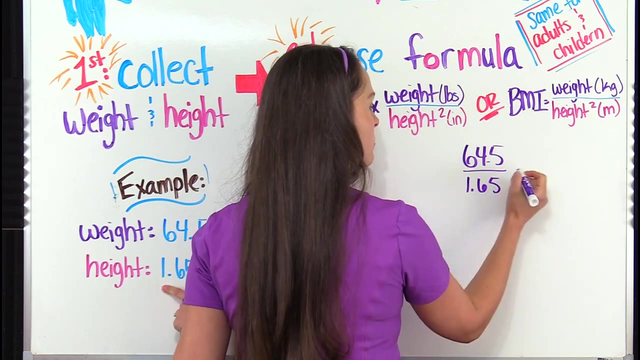 we're going to plug it in. so our patients weight in kilograms is 64.5, so 64.5. our height is in meters and they had a height of 1.65 meters and remember, don't forget to square. so we're going to. 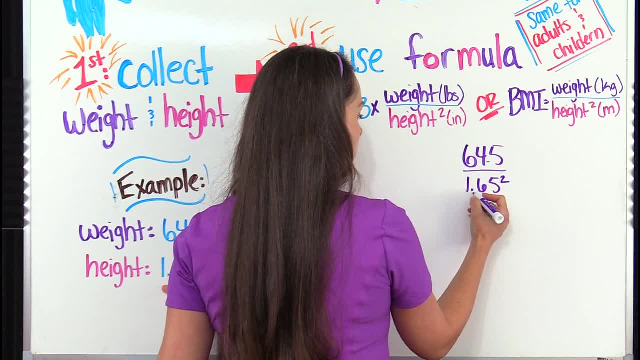 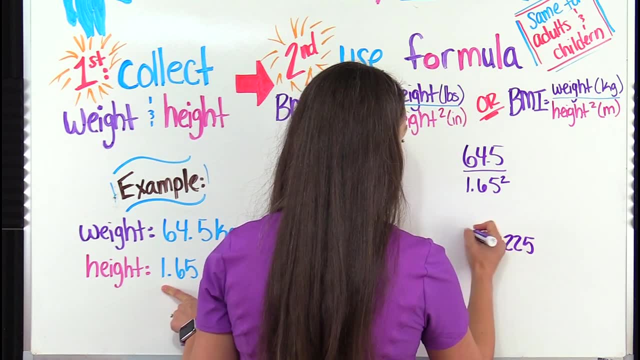 square it. so let's go ahead and do that. so we're going to square it. so we're going to square it. so ahead and square that out. so 1.65 squared gives us two point seven, two, two five, and we're going to bring down our sixty four point five and we're going to just divide that out. so whenever we